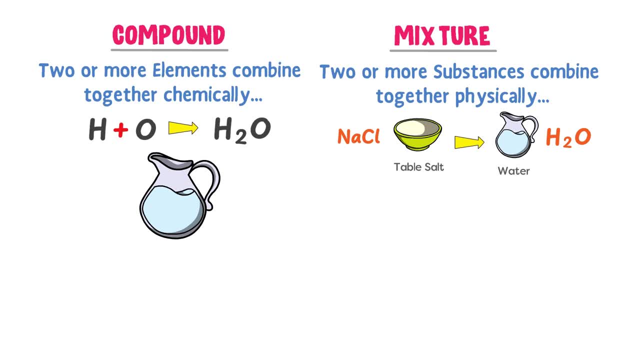 salt, NaCl and water. H2O are compounds When you dissolve table salt, NaCl and water. H2O are compounds When you dissolve table salt, NaCl and water. H2O are compounds When you dissolve table salt, NaCl and water. H2O are compounds When you physically mix copper and tin. 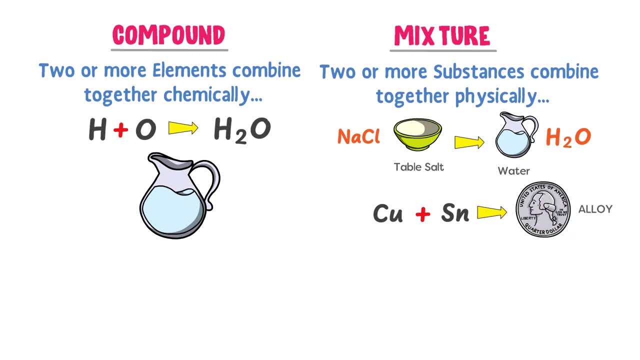 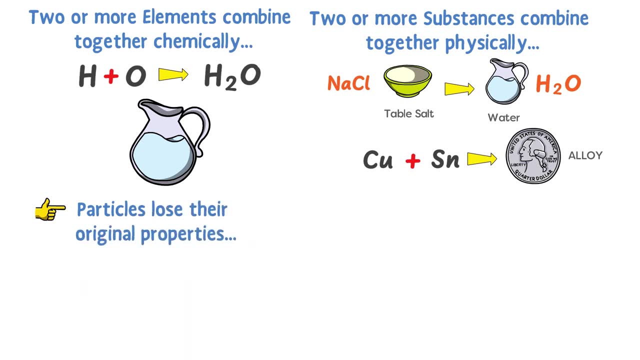 you get a mixture, also commonly known as alloy. Secondly, in compounds, particles lose their original properties. For example, hydrogen and oxygen are gases, But when they are combined together chemically, they form a compound. When you physically mix copper and tin, you get a 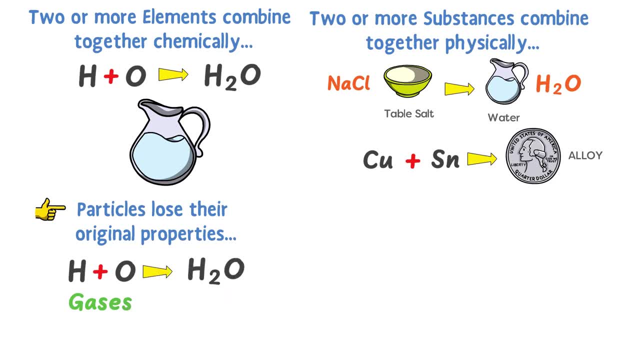 mixture, also commonly known as a mixture. But when they are combined together chemically they form a compound. They change back to their original properties. In these air and gas compounds their original properties change and become a new substance or water. In mixture particles. 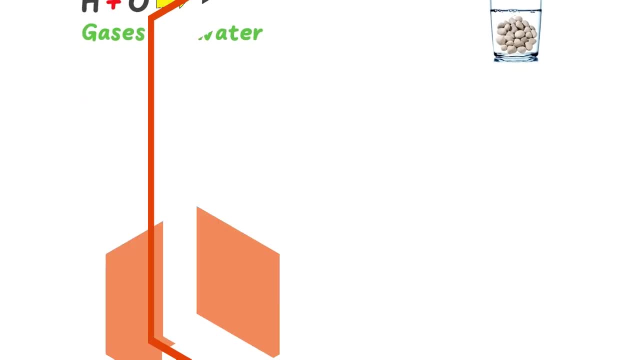 retain their original properties. For example, when you add some pebbles to the water, both the pebbles and the water retain their original properties. Thirdly, compound always has oxygen and hydrogen in the water. On the other side, mixture has either homogeneous or heterogeneous. 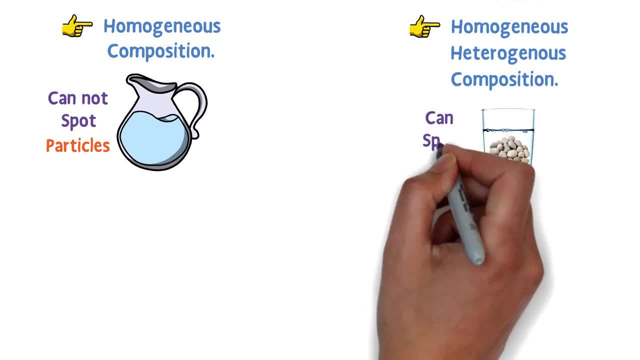 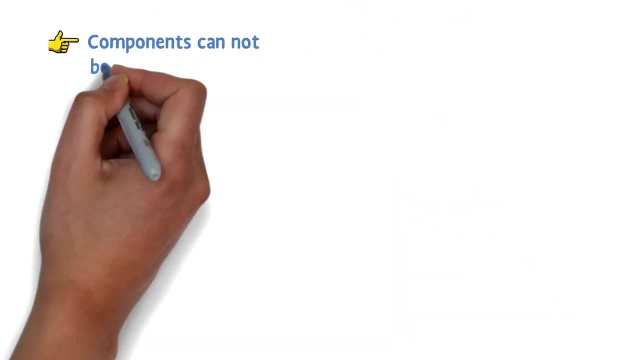 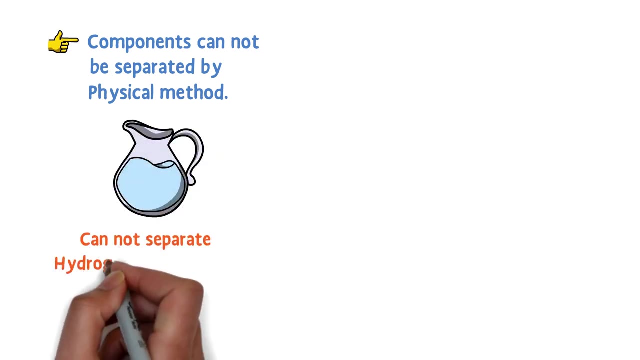 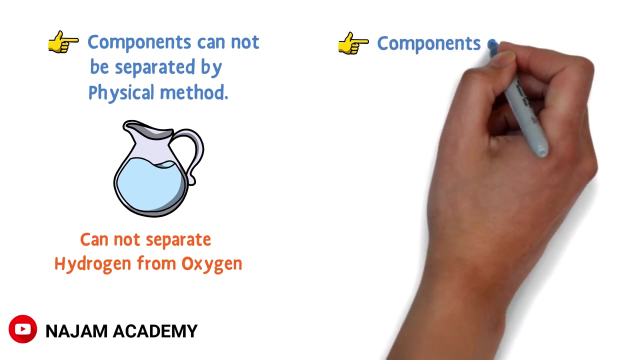 composition. For example, you can spot both pebbles and water in this mixture. Fourthly, components of the compound cannot be separated by any physical method. For example, you cannot separate hydrogen from oxygen in the water by any physical means, While components of the mixture 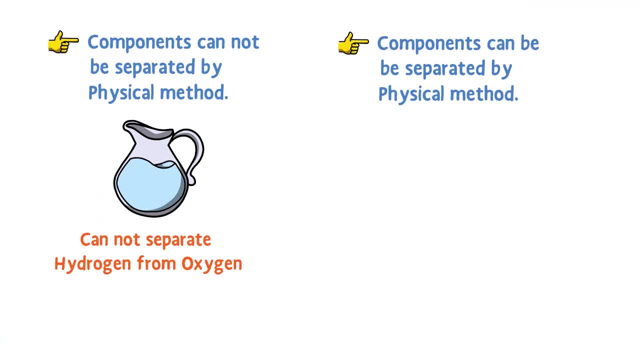 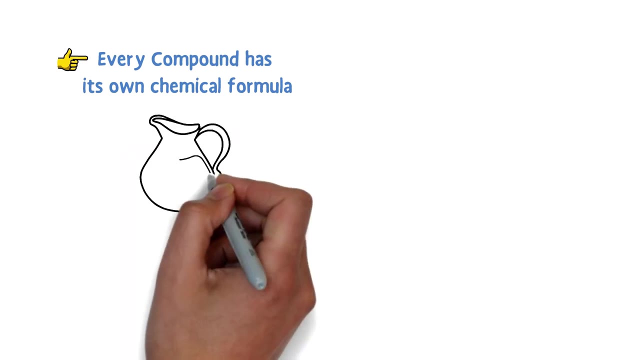